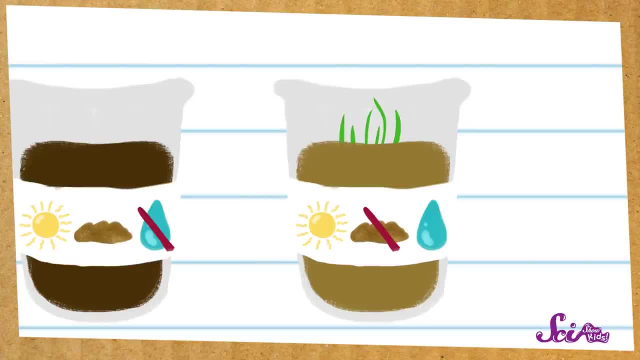 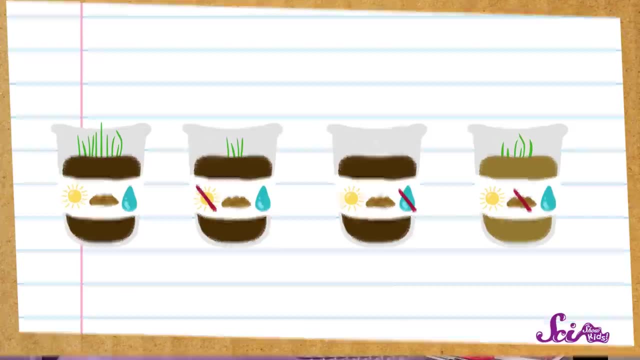 Also, I think the plant that's in sand will grow pretty well, since the plant can make its own food from sunlight. Now that we have our guesses about what will happen, we can prepare for our experiment. Let's get started. For our plants, we'll need four containers that you can cut a hole in. 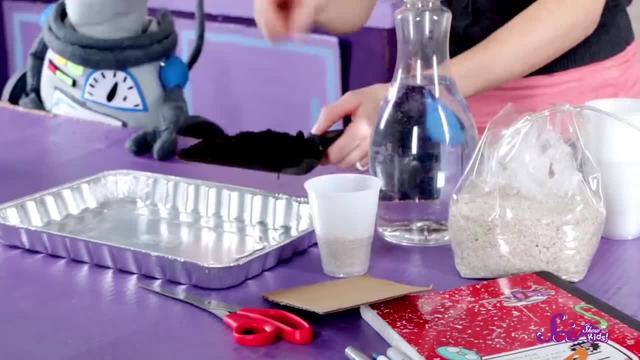 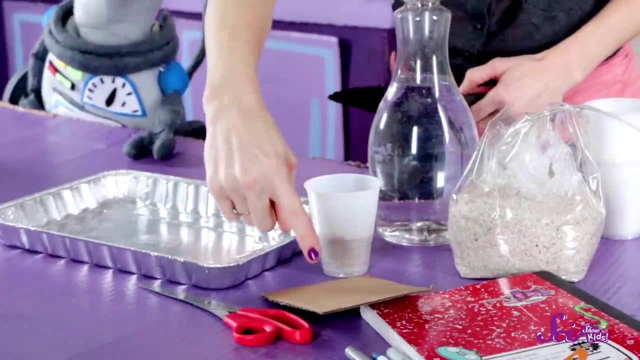 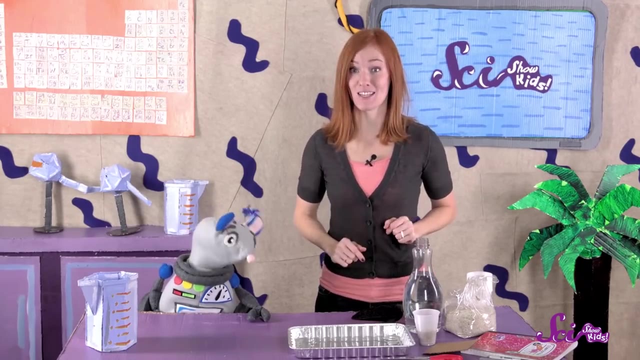 We're going to use small plastic cups. We'll also need soil, water, sand, seeds, a drain pan, a small cardboard square and scissors. You can use any seeds you like, but make sure to use the same kind of seeds for all of the. 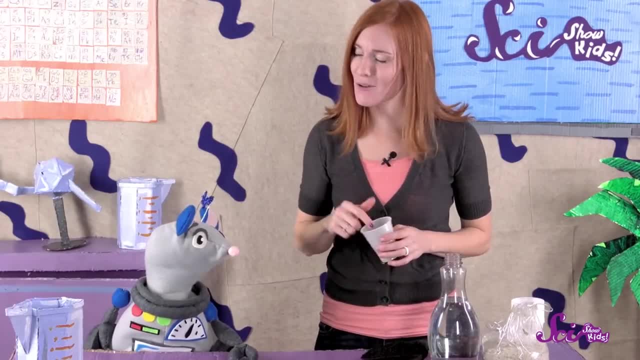 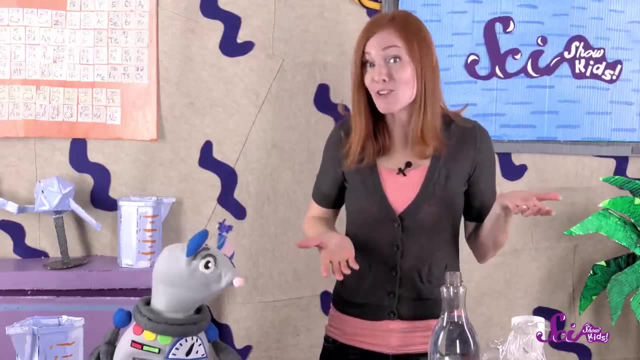 containers For this experiment. I found some extra grass seeds that we're going to use. Like Squeaks and I are doing. you can use a plant journal to track how your plants change. You can write down things like how tall the plants are and what color they are. 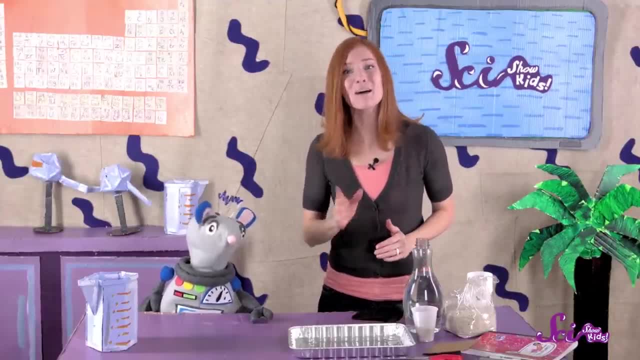 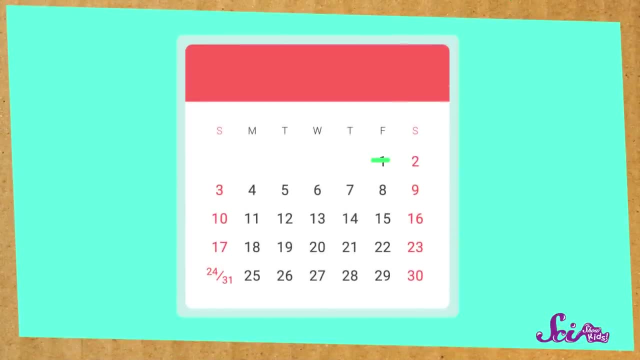 Also, something that's really fun to do is to take pictures of your plant, but if you don't have a camera to use, you can just draw what you see. Finally, you'll need a lot of time. Your plants could take a few weeks or even a month to grow. 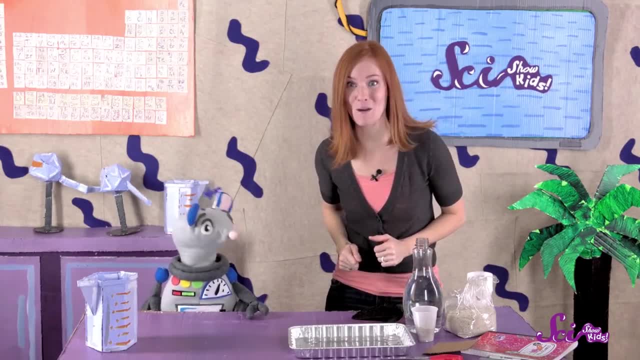 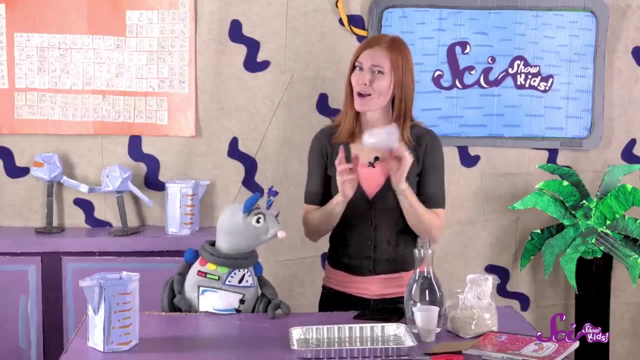 Alright, now that we have all the supplies, it's time to start our experiment. First, let's mark each cup with the things that the plant is missing and then cross that out On one cup. we won't draw anything. This cup will be for the seeds that get empty. 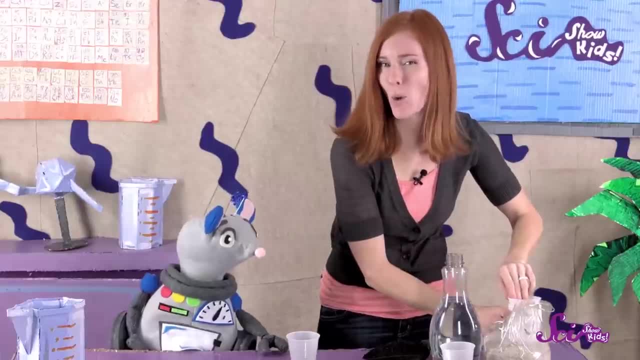 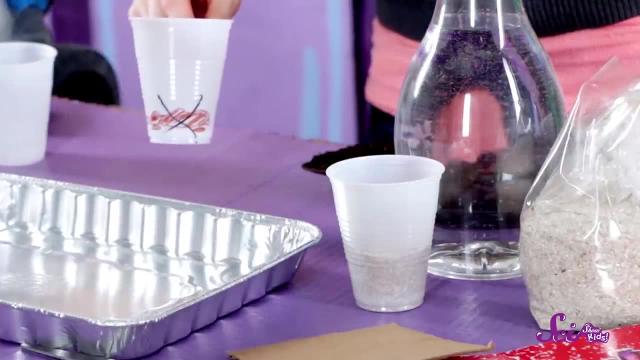 For the second cup, let's draw soil, then X over it to cross it out. These seeds will get sunlight and water, but there will be sand in the cup instead of soil. On the next cup, let's draw a sun and again cross that out. 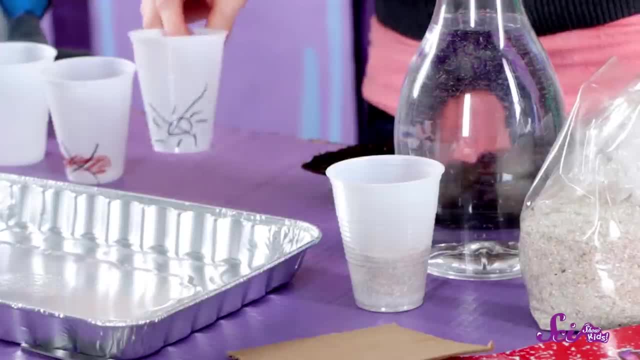 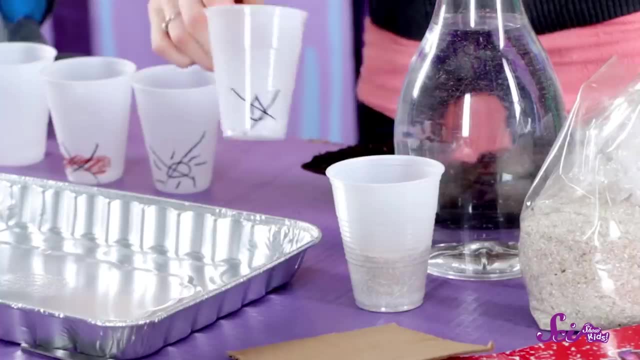 These seeds will get water and soil, but no sunlight. Okay, here's the last cup For this one. we'll draw a water droplet and then cross that out. These seeds will have good soil and get plenty of sunlight, but no water. 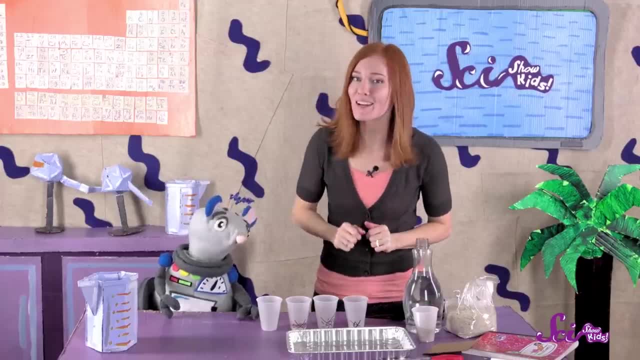 Now that we've marked each cup with the things that the plant is missing, let's start our experiment. First, our four cups. We'll make a small hole in the bottom of each cup. Ask for help from a grown-up for this step. 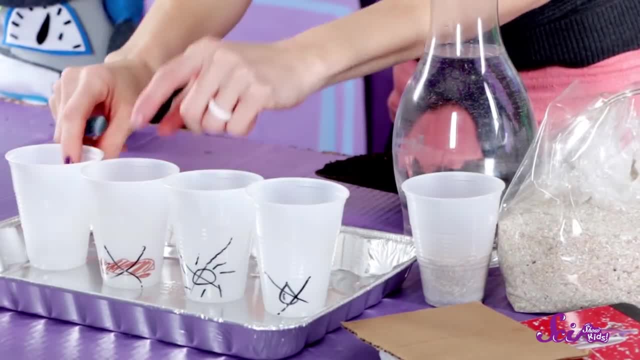 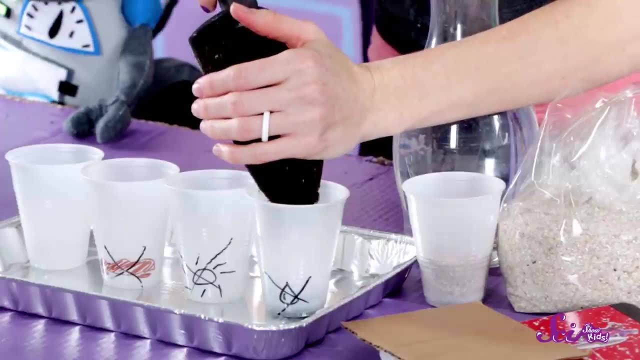 And now it's time to put each cup in the pan and fill them up. We'll fill one cup with sand and all the other cups with soil, But don't fill up the cups all the way. We'll need to leave some room for when we water our seeds.